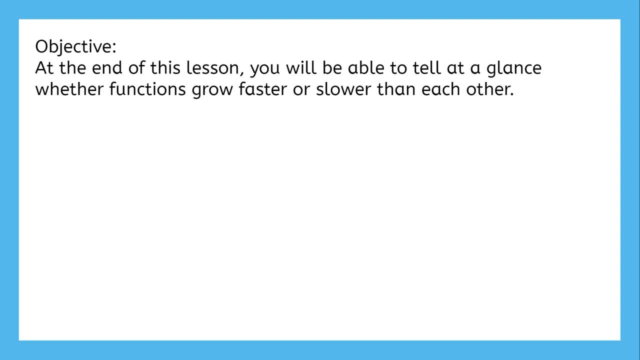 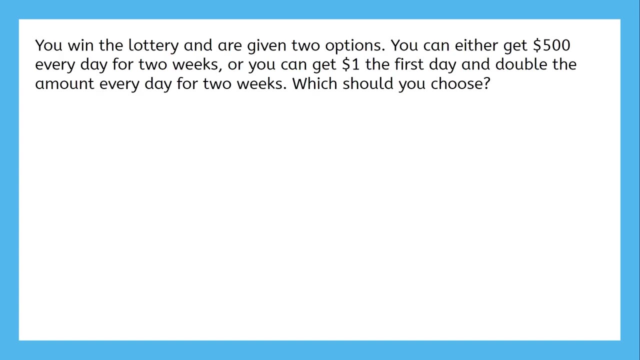 tell at a glance whether functions grow faster or slower than each other. First we will take a look at two examples comparing linear and exponential growth functions. then we'll compare three different exponential growth functions to each other. You win the lottery and are given. 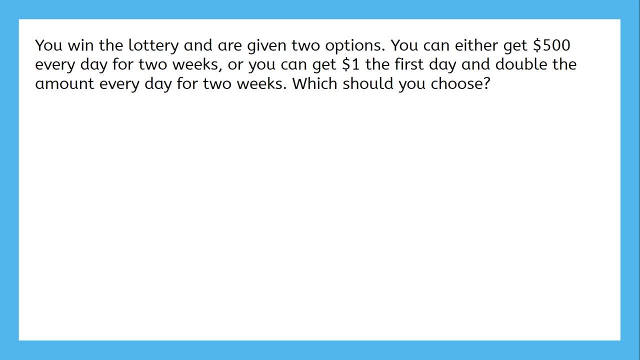 two options. You can either get $500 every day for two weeks, or you can get $1 the first day and double that amount every day for two weeks. Which should you choose? For the first option, you receive $500 at first, then add another 500 dollars thirteen more times, resulting in a linear. 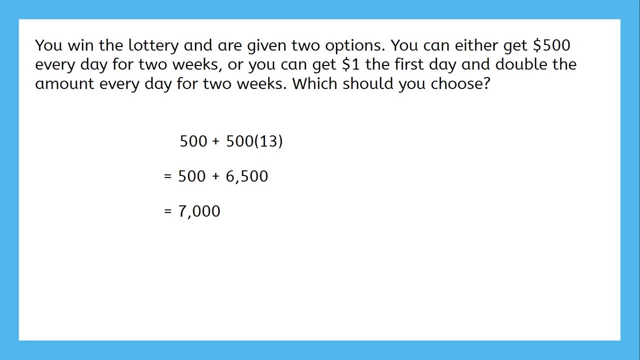 expression that totals $7,000.. In the second option, you start with only $1,, but then it doubles 13 times, creating an exponential expression equaling $8,192.. So the exponential option, despite how bad it first sounded, actually ended up being the better one. But how? 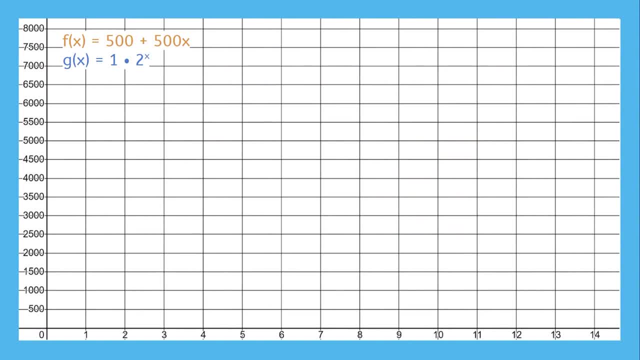 Let's compare the two functions over time by graphing them. In the beginning, the first option started at 500, and the second option started at 1.. The next day, the first option adds 500 more, while the second option only goes up to 2.. This gap is just getting wider There. 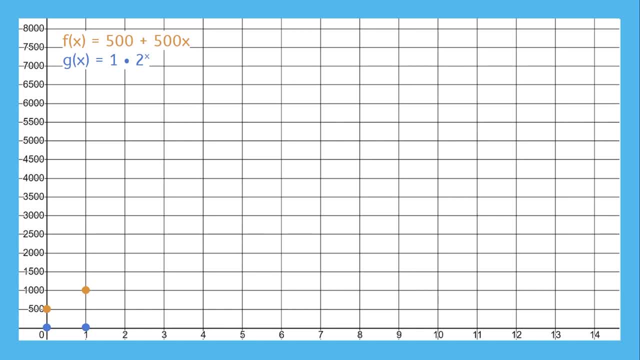 is no way. the second option was better. But if we finish graphing both functions, something interesting happens. For the first few days, the exponential function didn't seem to be going anywhere, But then, starting at about day 6, it started increasing. 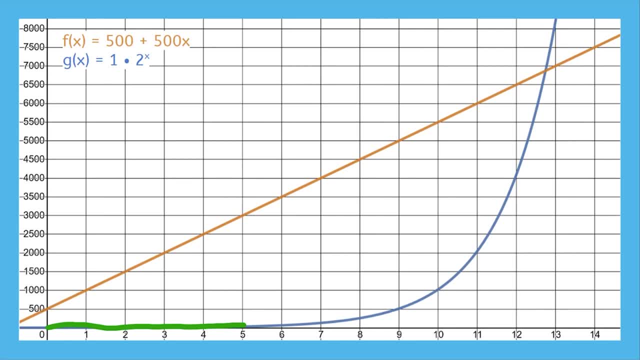 faster and faster. On the 10th day the exponential function has sped up so much that it gains $512, more than the linear function gains on any day, And the exponential option just keeps speeding up. If you are only receiving money for 13 days, the first option- 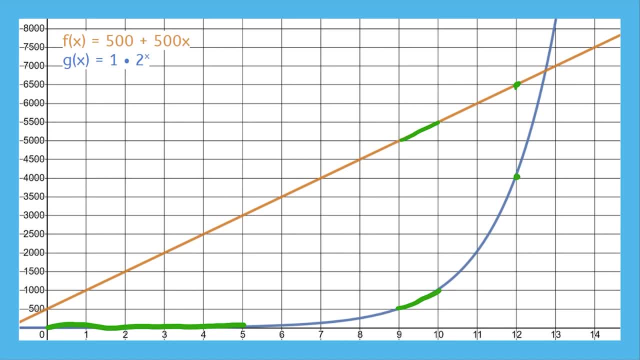 would have been about $2,500 better, But on the very last day the exponential option gains enough to pull ahead of the linear option by over $1,000.. This will always happen when comparing exponential functions to linear functions. Eventually, the exponential function will 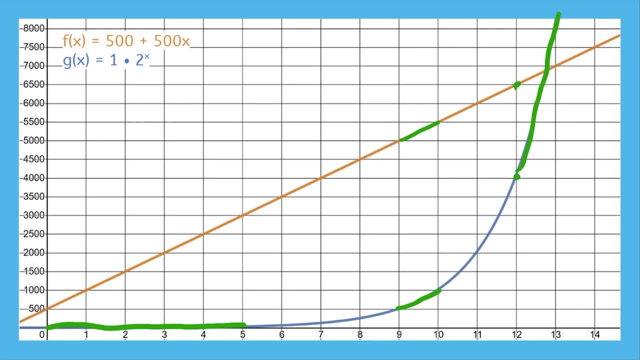 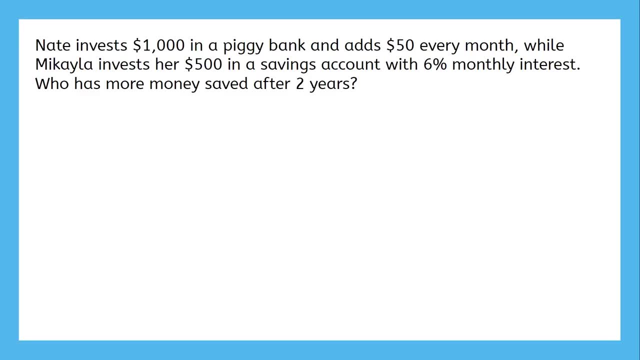 outpace the linear one. It's not a question of whether the exponential function will surpass the linear function. It's about when Nate invests $1,000 in a piggy bank and adds $50 to it every month, while Mikayla invests. 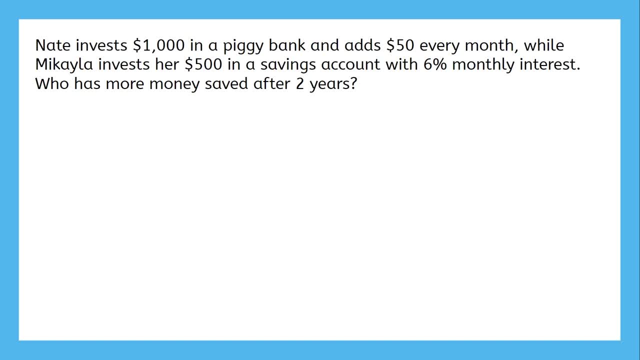 her $500 in a savings account with 6% monthly interest. Who has more money saved after two years? So Nate starts with $1,000 and adds $50 to it every month, And Mikayla only invests $500, but receives 6% interest every month. 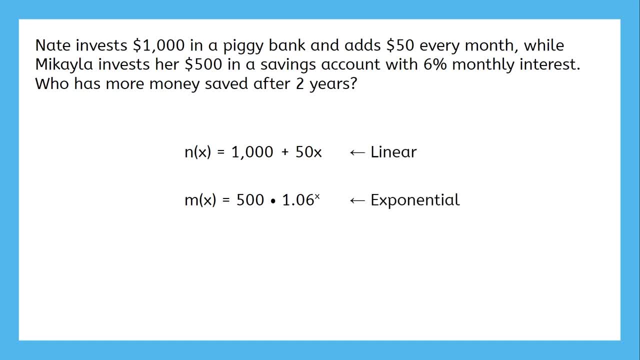 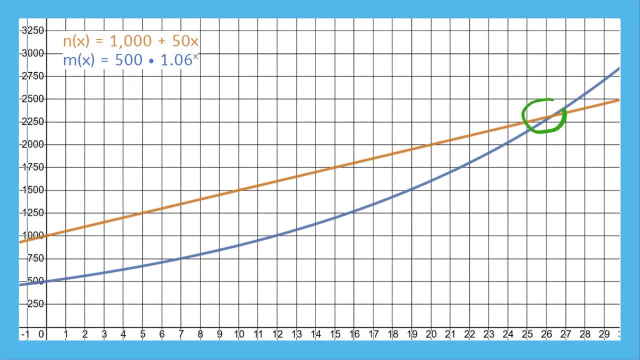 So, just like last time, we're comparing a linear function to an exponential function. Does this mean Mikayla's exponential savings account automatically wins? Not necessarily. If we graph both functions, we can see how they compare over time. Like we said before, 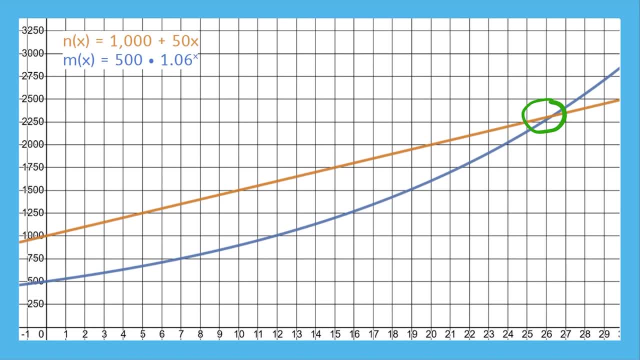 an exponential function will always speed past a linear function. But we were asked a specific question: How do they compare after two years? That's the initial amount plus 23 more months. So we look where the input is 23.. And at that. 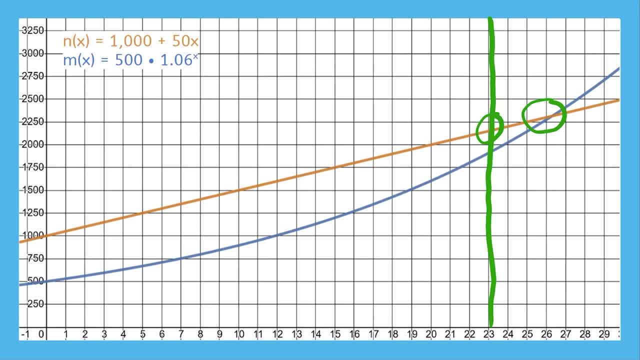 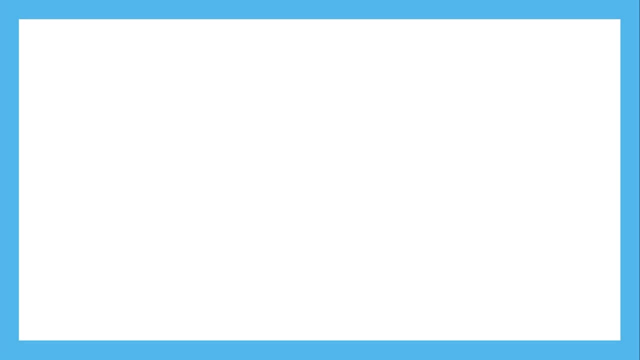 point. the linear function is still higher, So Nate would have more money saved after two years. It'll take another four months for Mikayla's savings account to pass Nate's piggy bank. Even though this video is about comparing linear and exponential functions, it's also 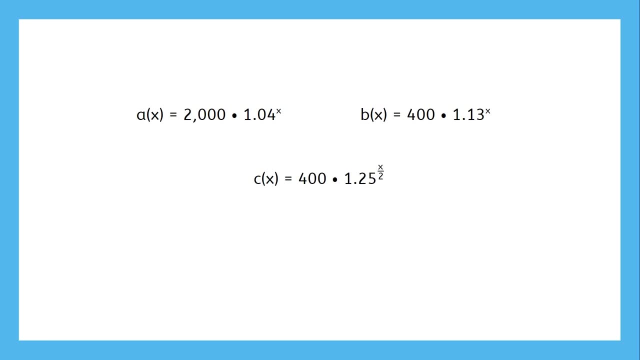 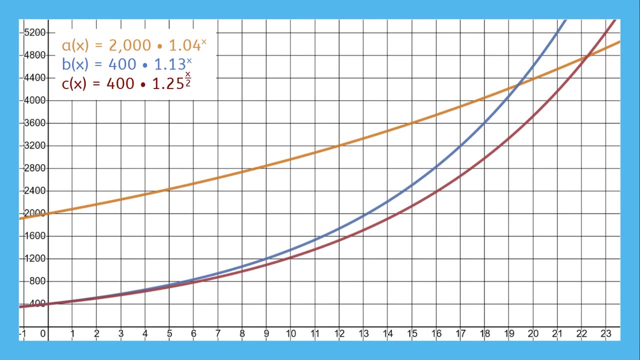 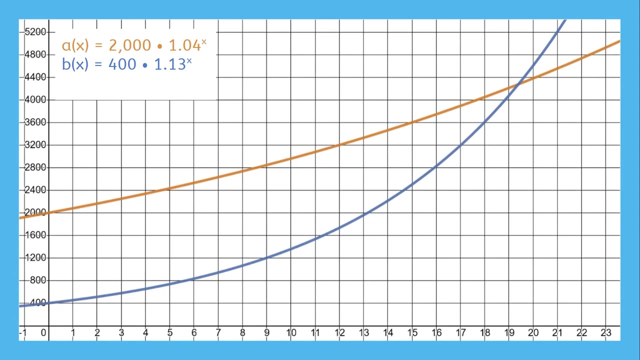 important to understand how exponential functions compare. We can graph all three of these and see that some of them move nice and slow, while others speed by. If we compare functions A and B, we see that B outpaces A at around the input 19.5 mark. 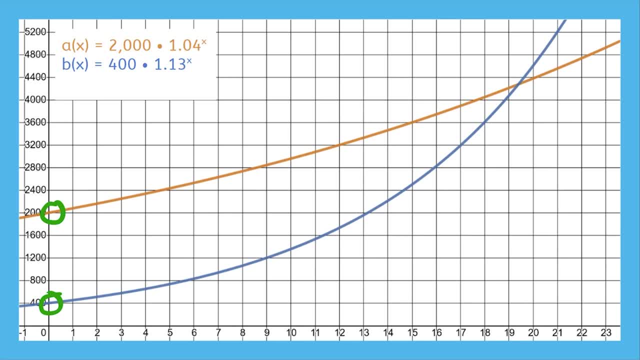 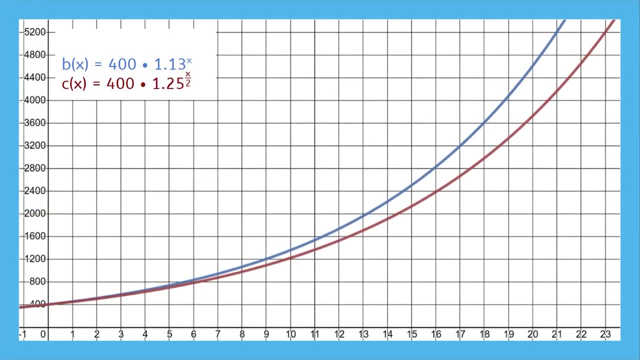 despite the huge lead A had at the beginning. Why is that? It's because B has a higher growth factor. Higher growth factors will always grow faster than smaller growth factors. If we compare functions B and C, C seems to have a higher growth factor, Yet B comes out. 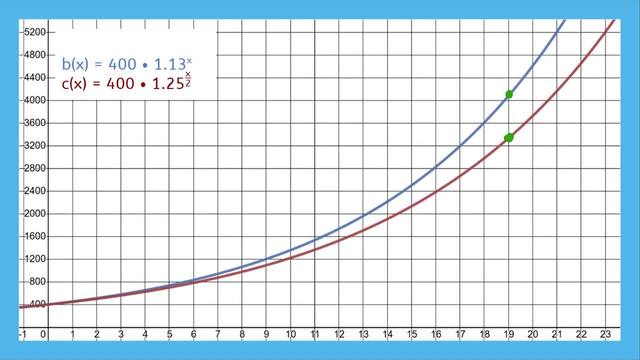 ahead. This is because C's growth factor occurs every two units. To get a better idea of how quickly it grows, we can rewrite the exponent's denominator as a root. This way, we can clearly see that B has a slightly higher growth factor, meaning it will end up higher. 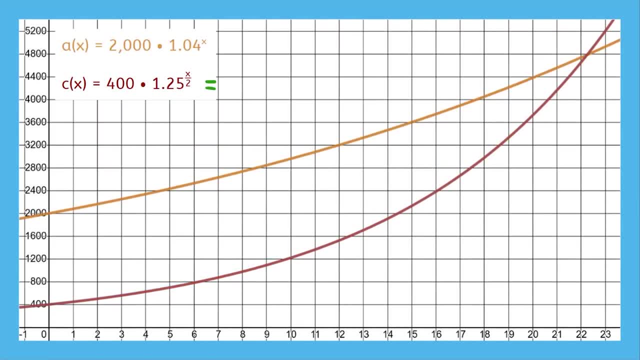 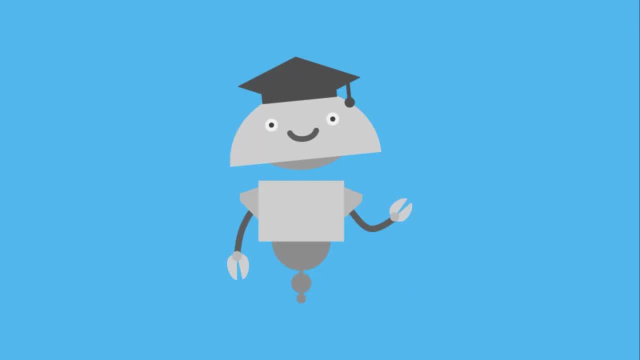 than C And, of course, now that we know the true growth factor of function C, we can see why it surpasses function A. Keep these basic concepts in mind. Exponential functions always surpass linear functions eventually, and exponential functions with higher growth factors grow faster. 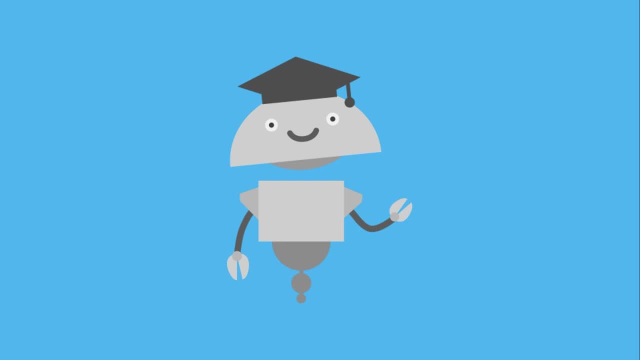 In the next lesson we'll learn about a different kind of exponential function: exponential decay. See you then. 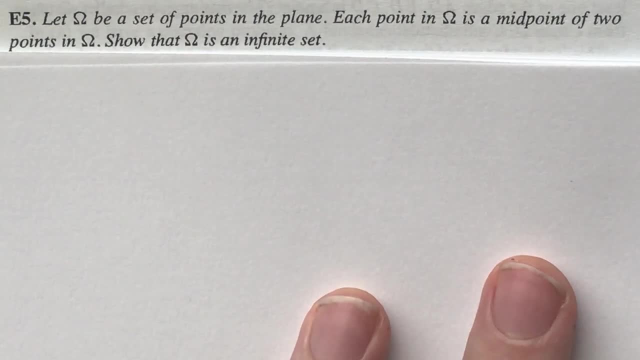 Hello fellow problem solvers. So today we're going to be doing a problem from Engel's problem solving strategies, Example number five in the extremal principle, Let's say introductory problem. first lesson in the extremal principle, which really says that whenever you have a problem and you're looking at some objects, pick an object with the biggest or smallest property of some kind. This problem I invite you to try out for a minimum of five minutes, ideally 10 to 15, but not more than an hour, And if, on the other hand, you'd like to go a lot, 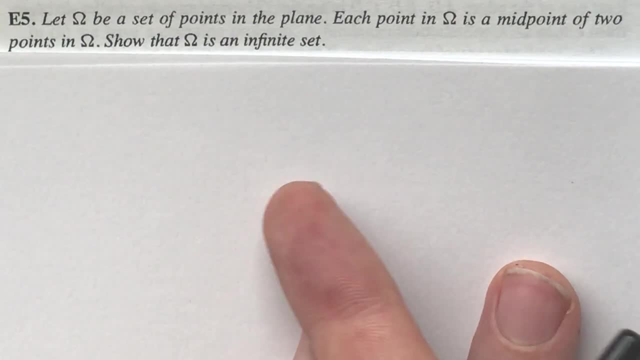 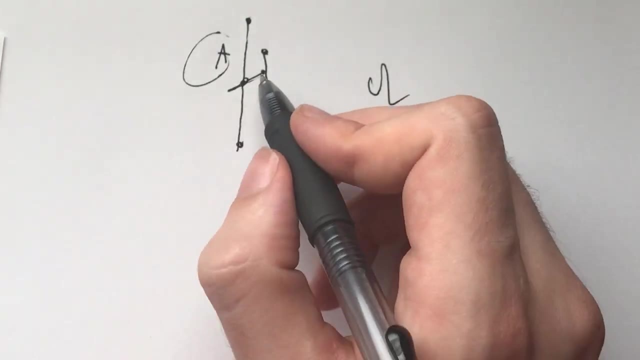 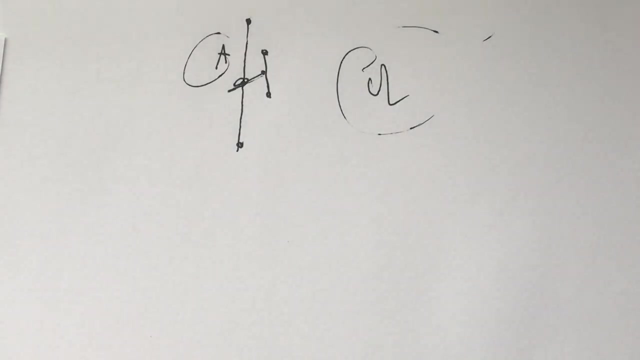 longer just read the problem and put your first idea or two out on paper and solve it really. So now let's begin. So this is what we have. We have this set such that any point in the set is a midpoint of two other, of a line segment connecting two other points from the same set, And how. we need to prove that this set is actually infinite. This is omega. And how would you do this? Well, like, okay, if a point is somewhere in the set.